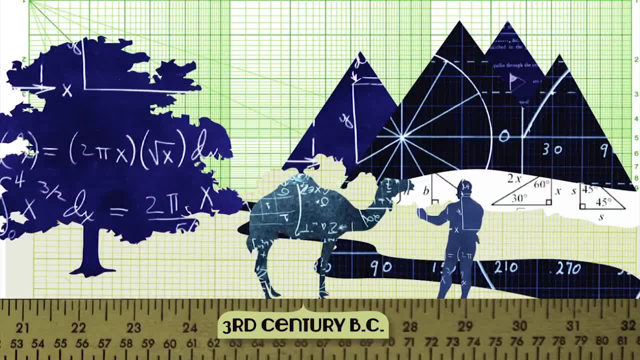 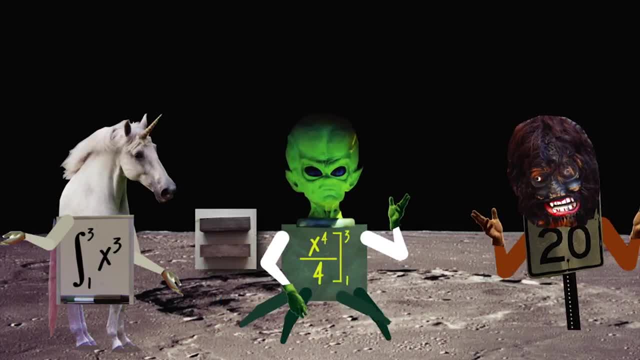 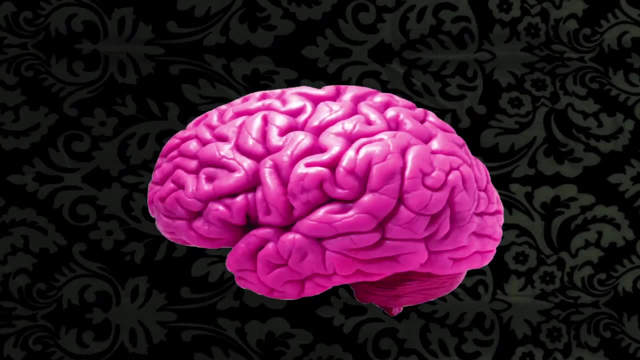 believed nature itself was the physical manifestation of mathematical laws. Others argue that, while numbers may or may not exist physically, mathematical statements definitely don't. Their truth values are based on rules that humans created. Mathematics is thus an invented logic exercise with no existence outside mankind's conscious thought. 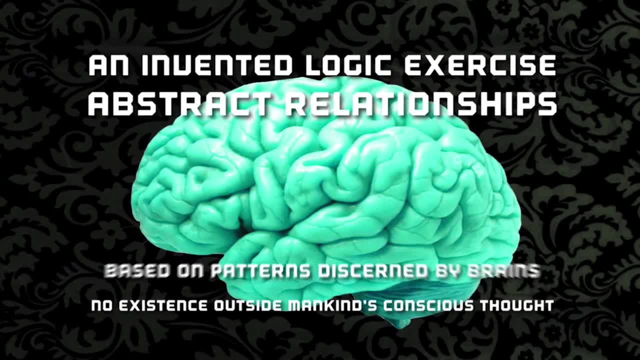 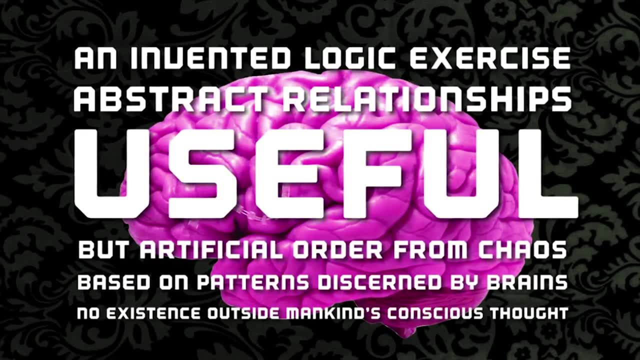 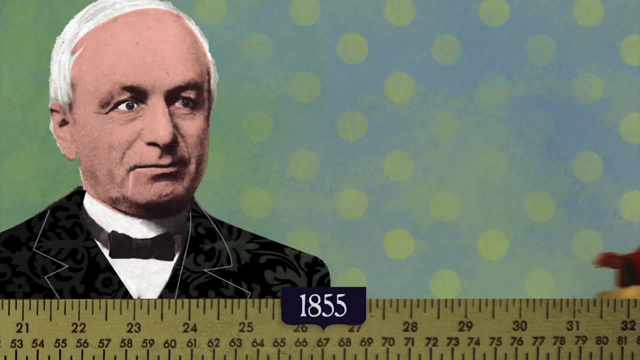 a language of abstract relationships based on patterns discerned by brains built to use those patterns to invent useful but artificial order from chaos. One proponent of this sort of idea was Leopold Kronecker, a professor of mathematics in 19th century Germany. 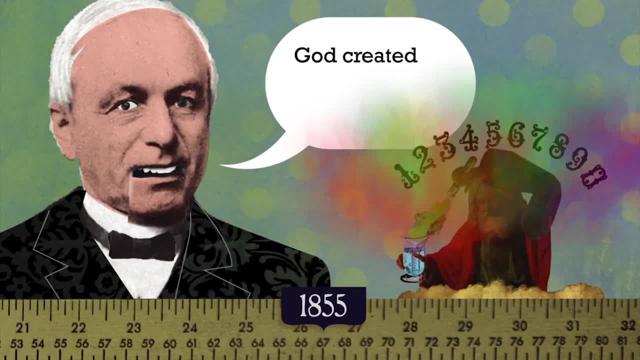 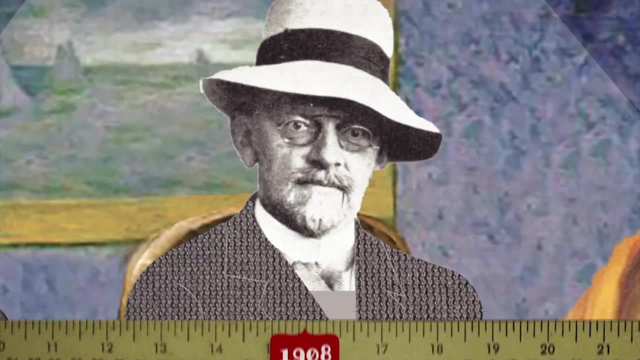 His belief is summed up in his famous statement: God created the natural numbers. All else is the work of man. During mathematician David Hilbert's lifetime, there was a push to establish mathematics as a logical construct. Hilbert attempted to axiomatize all of mathematics. 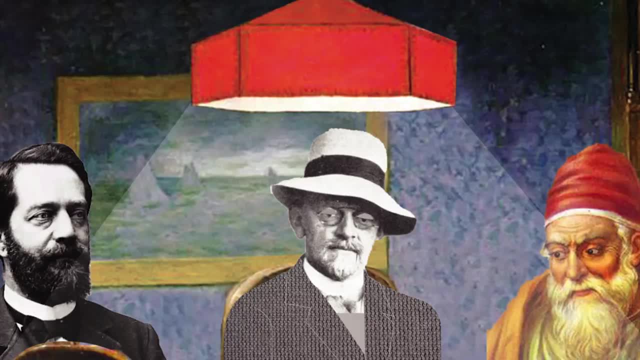 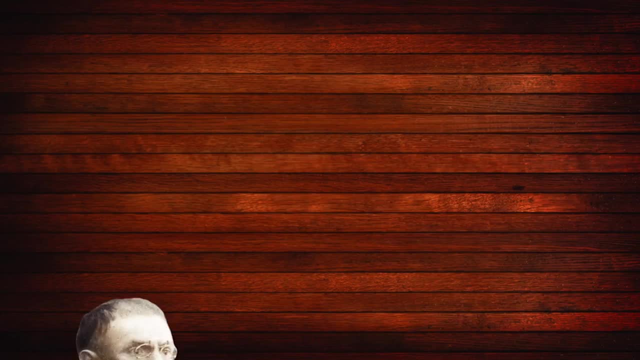 as Euclid had done with geometry. He and others who attempted this, saw mathematics as a deeply philosophical game, but a game nonetheless. Henri Poincaré, one of the fathers of non-Euclidean geometry, believed that the existence of non-Euclidean geometry 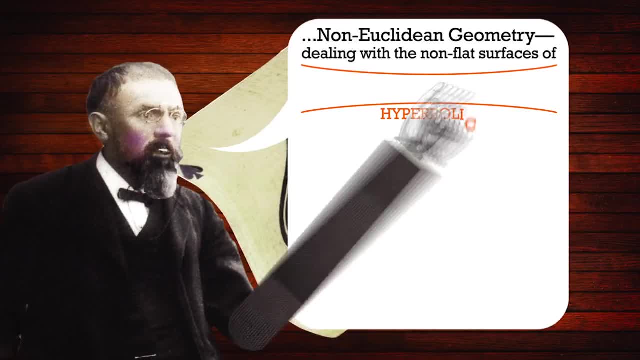 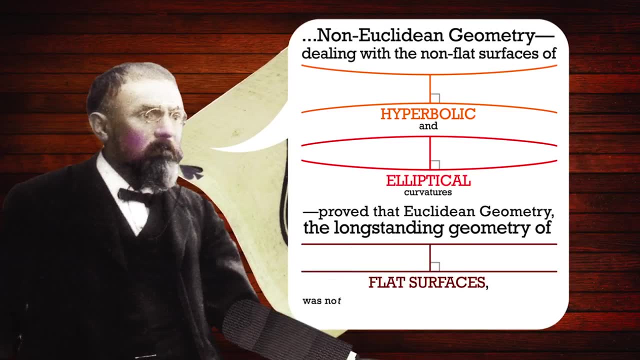 dealing with the non-flat surfaces of hyperbolic and elliptical curvatures proved that Euclidean geometry, the long-standing geometry of flat surfaces, was not a universal truth, but rather one outcome of using one particular set of game rules. But in 1960,, 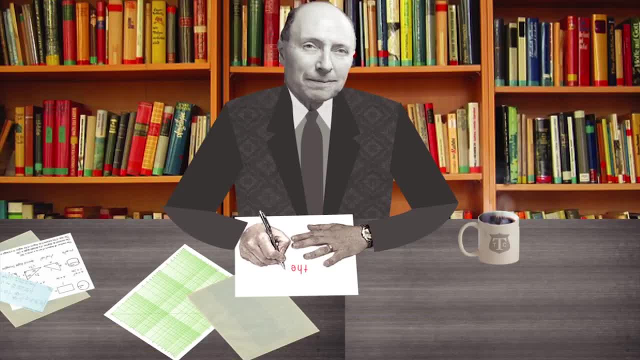 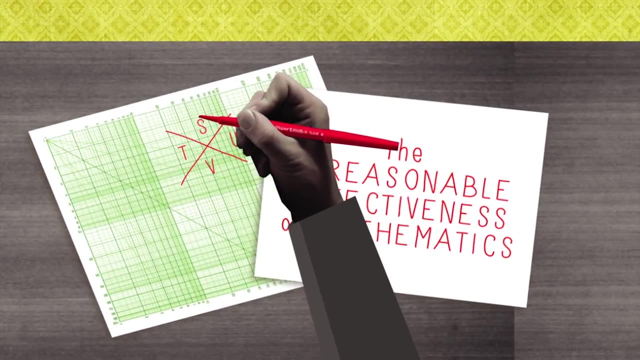 Nobel physics laureate Eugene Wigner coined the phrase the unreasonable effectiveness of mathematics. pushing strongly for the idea that mathematics is real and discovered by people, Wigner pointed out that many purely mathematical theories developed in a vacuum, often with no view towards describing any physical phenomena. 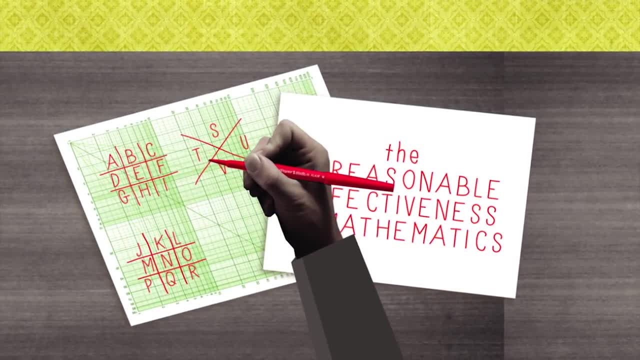 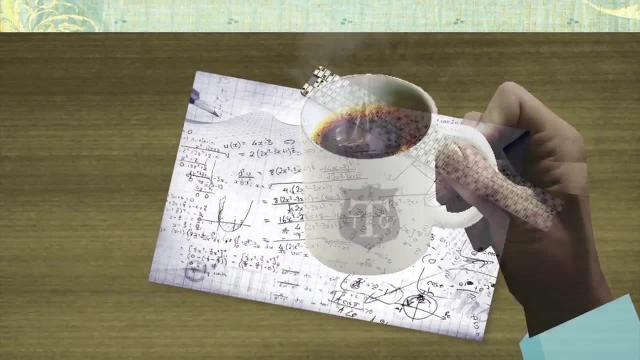 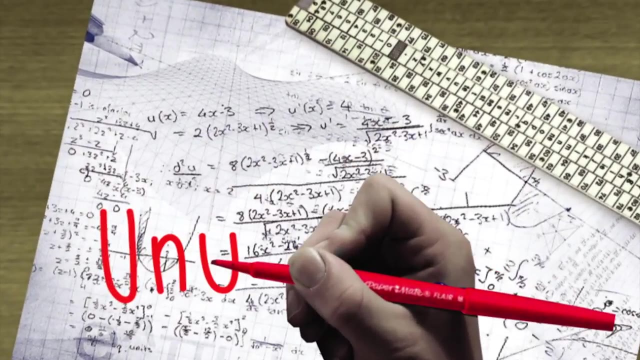 have proven, decades or even centuries later, to be the framework necessary to explain how the universe has been working all along. For instance, the number theory of British mathematician Godfrey Hardy, who had boasted that none of his work would ever be found useful in describing any phenomena in the real world. 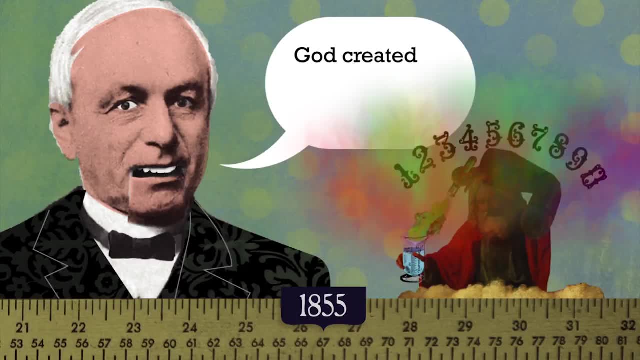 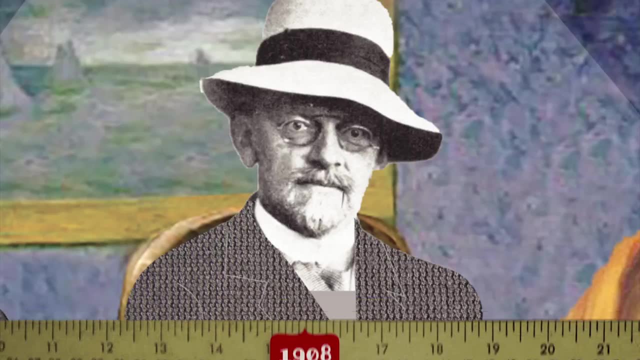 His belief is summed up in his famous statement: God created the natural numbers. all else is the work of man. During mathematician David Hilbert's lifetime, there was a push to establish mathematics as a logical construct. Hilbert attempted to axiomatize all of mathematics. 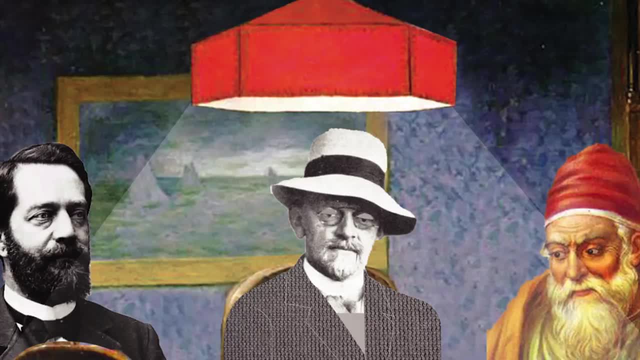 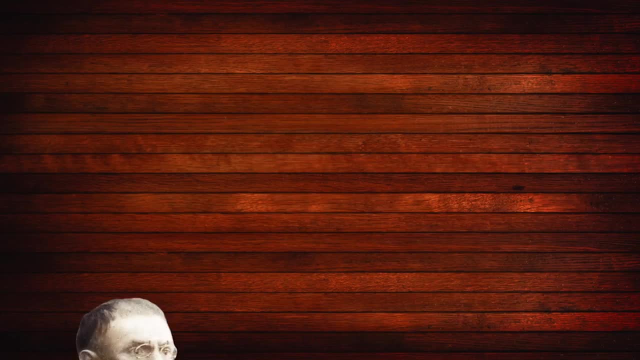 as Euclid had done with geometry. He and others who attempted this, saw mathematics as a deeply philosophical game, but a game nonetheless. Henri Poincaré, one of the fathers of non-Euclidean geometry, believed that the existence of non-Euclidean geometry 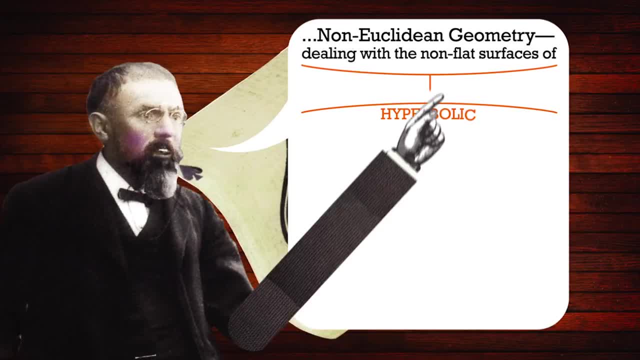 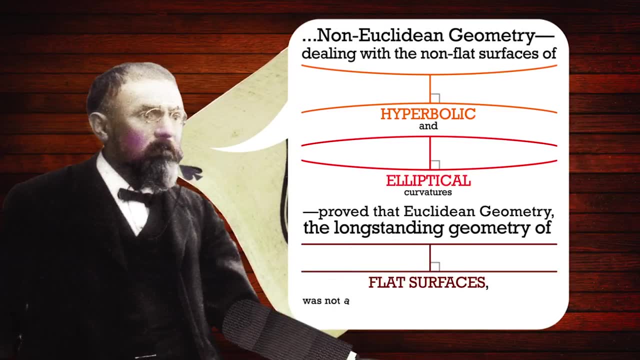 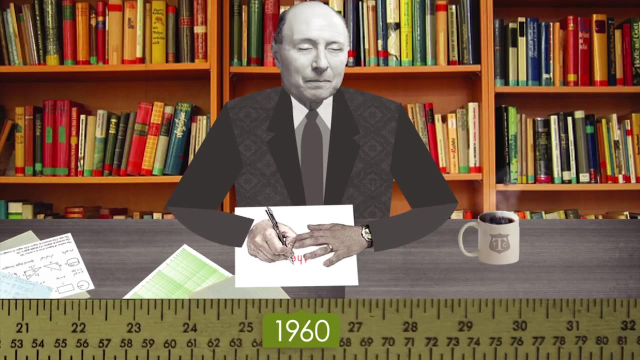 dealing with the non-flat surfaces of hyperbolic and elliptical curvatures proved that Euclidean geometry, the long-standing geometry of flat surfaces, was not a universal truth but rather one outcome of using one particular set of game rules. But in 1960, Nobel physics laureate Eugene Wigner 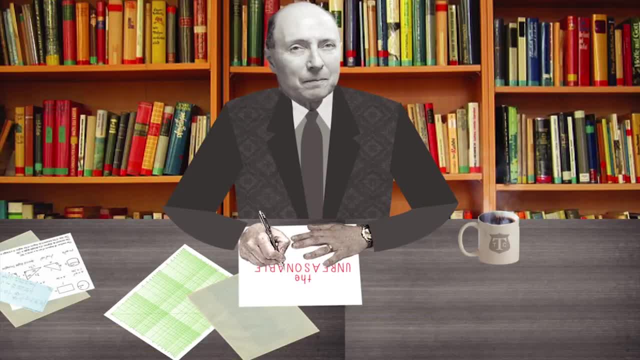 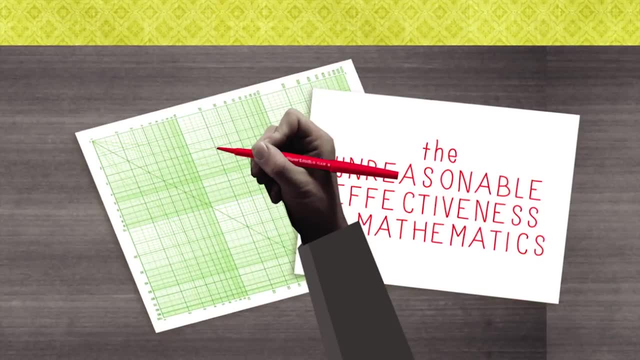 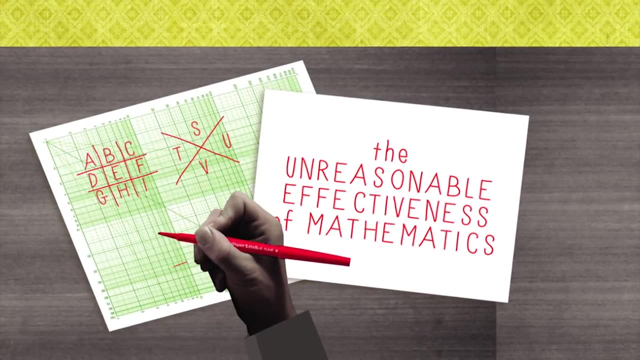 coined the phrase- the unreasonable effectiveness of mathematics. pushing strongly for the idea that mathematics is real and discovered by people, Wigner pointed out that many purely mathematical theories developed in a vacuum, often with no view towards describing any physical phenomena, have proven decades or even centuries later. 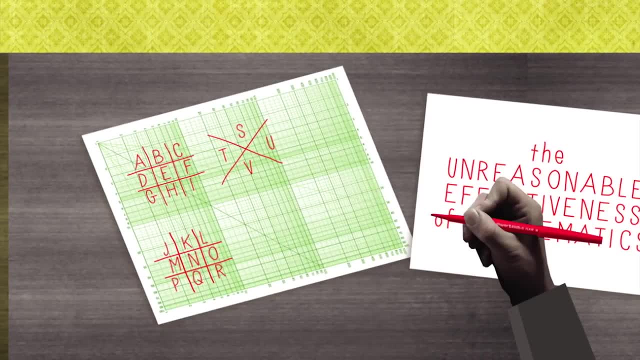 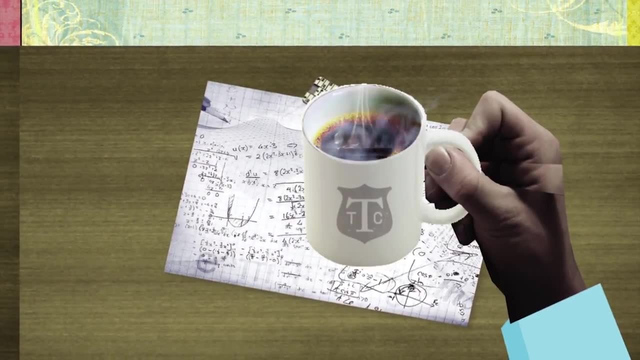 to be the framework necessary to explain how the universe has been working all along, For instance, the number theory of British mathematician Godfrey Hardy, who had boasted that none of his work would ever be found useful in describing any phenomena in the real world. 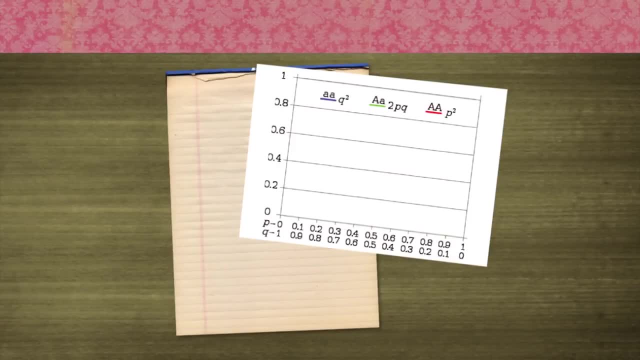 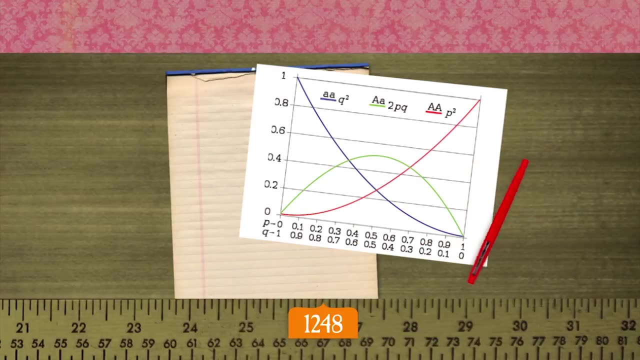 helped establish cryptography, Another piece of his purely theoretical theory. the work of Einstein became known as the Hardy-Weinberg law in genetics and won a Nobel Prize. And Fibonacci stumbled upon his famous sequence while looking at the growth of an idealized rabbit population. 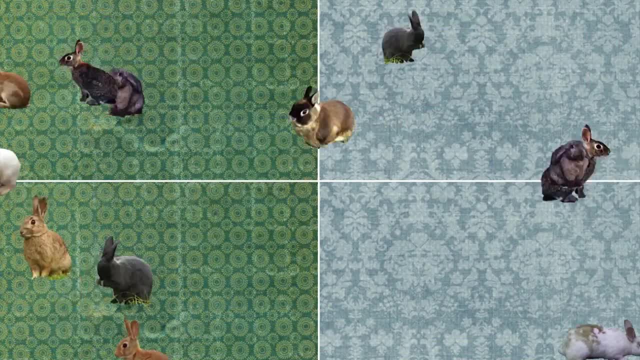 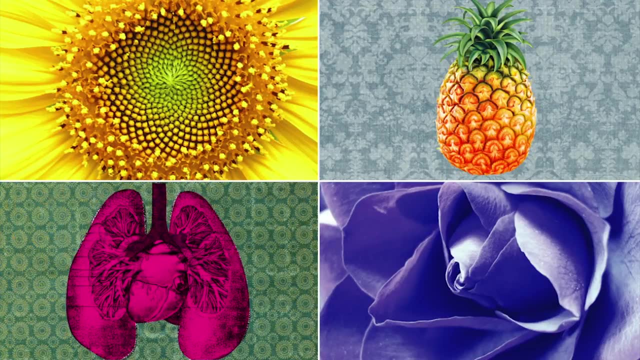 Mankind later found the sequence everywhere in nature, from sunflower seeds and flower petal arrangements to the structure of a pineapple, even the branching of bronchi in the lungs. Or there's the non-Euclidean work of Bernhard Riemann in the 1850s. 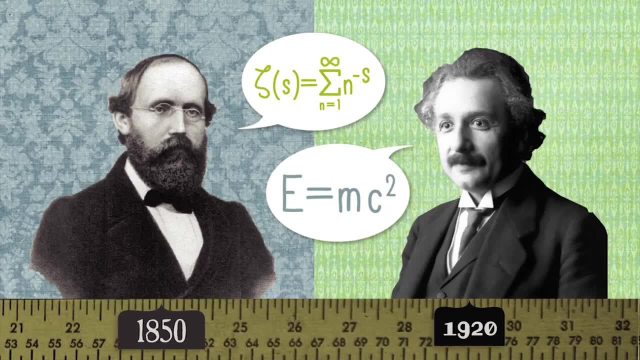 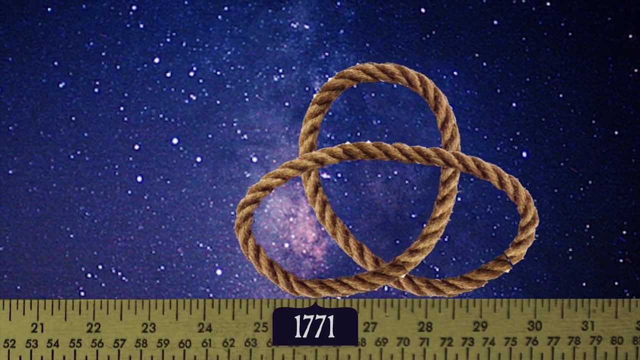 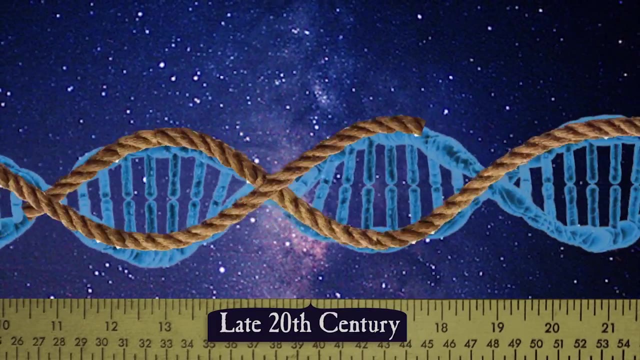 which Einstein used in the model for general relativity a century later. Here's an even bigger jump. Mathematical knot theory, first developed around 1771 to describe the geometry of position, was used in the late 20th century to explain how DNA unravels itself during the replication process.